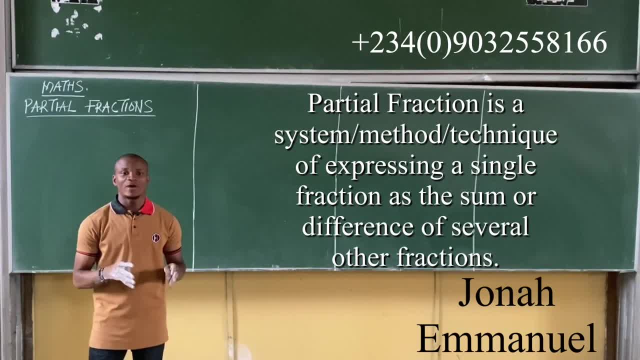 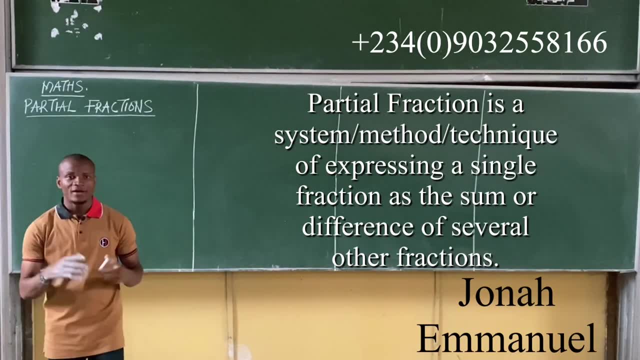 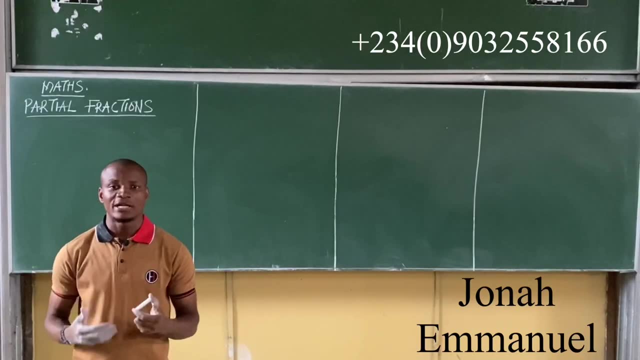 I'll be given a single fraction and I'll be asked to express that fraction as either the sum or the difference of several other fractions. When it comes to solving problems on partial fractions, there are certain rules that you must follow. So if you look at these rules, one after the other. 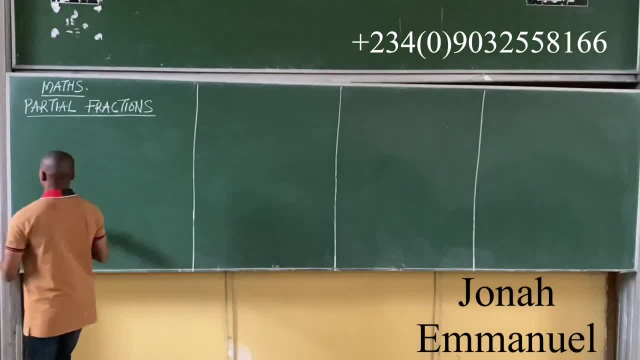 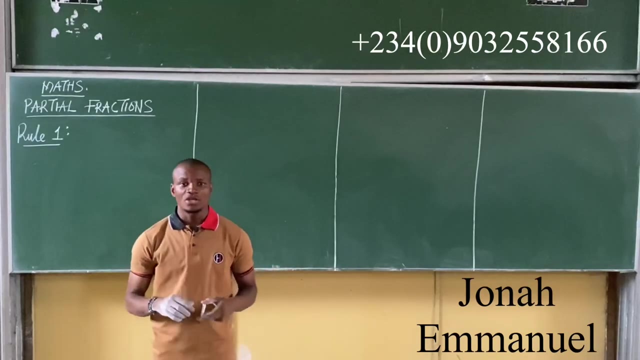 Let's look at the first rule. It's called rho-1. So what's the first rule to look out for when it comes to solving problems on partial fractions? Let's consider rho-1. Rho-1 says that if the form or if the factors of the denominator are linear in the form ax plus v. 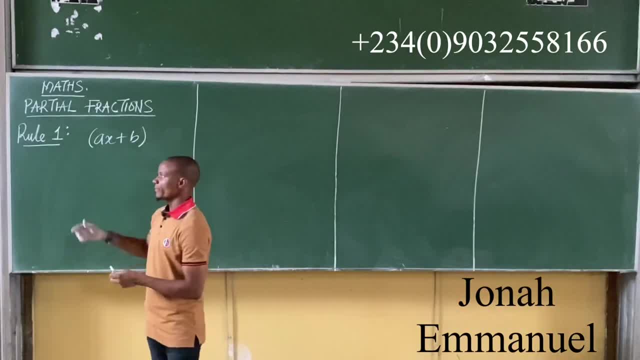 of denominator are linear in the form AX plus B, then a partial fraction of the form A all over AX plus B exists. 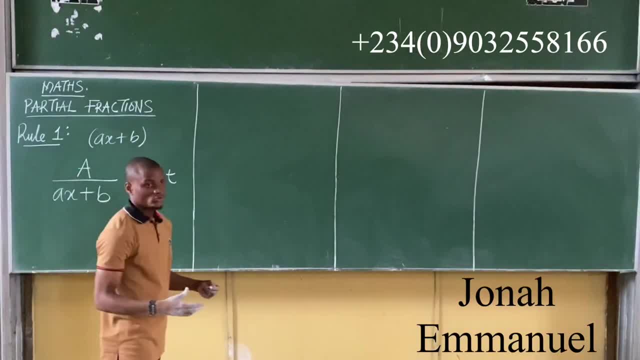 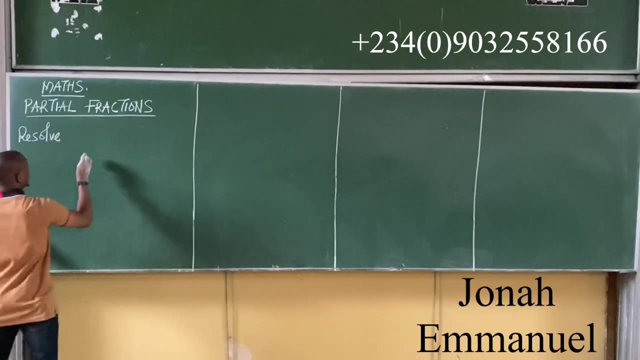 Alright, so we have it. We will take an example to further explain this point. Alright, for our first example, example 1, let's resolve 1 all over X squared plus 5X plus 6 into partial fraction. Alright, let's consider this example. 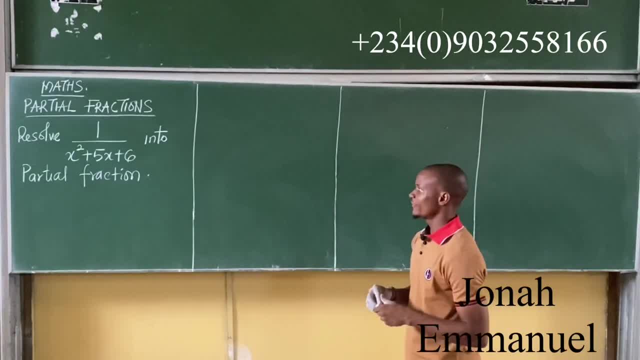 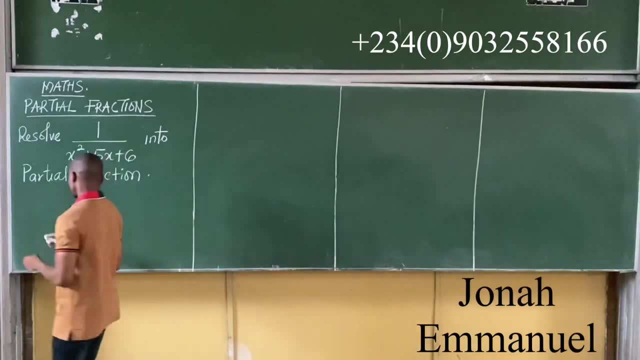 So here we have to resolve 1 all over X squared plus 5X plus 6 into partial fraction. Solution to this, now whenever it comes to solving problems on partial fraction, your first task is to consider the denominator. 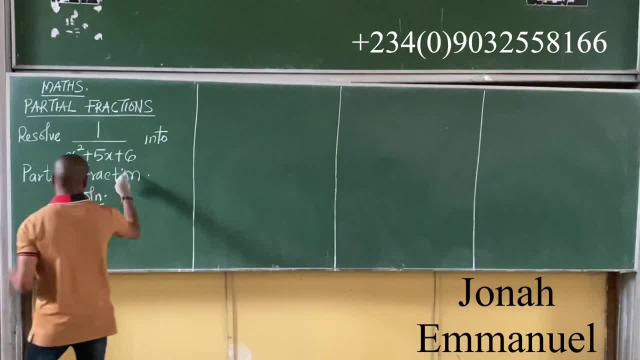 In this case here, my denominator is this. In this case, the denominator here is X squared plus B. Plus 5X plus 6. 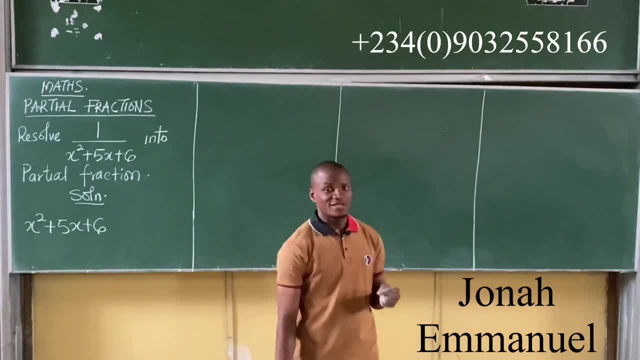 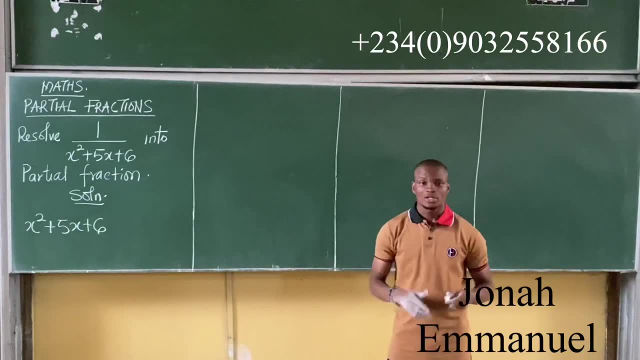 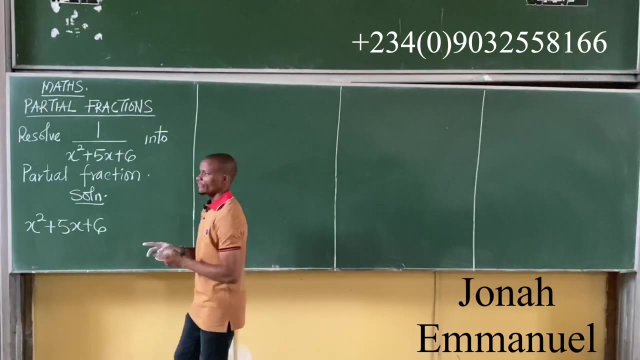 Now, observe that the denominator is quadratic in nature. H being quadratic means it will have two roots. So my first task is to find the two roots of this quadratic denominator. That means I will look for two numbers such that if these two numbers add up, they will give you 5. And if they multiply, they will give you 6. The numbers are plus 2 and plus 6. Plus 3. If I add 2 and 3, both be positive, I will have 5. If I multiply 2 and 3, I will have 6. 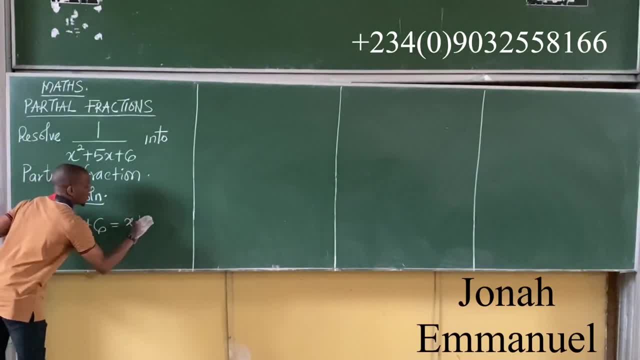 So this is going to be equal to X plus 2 into X plus 3. 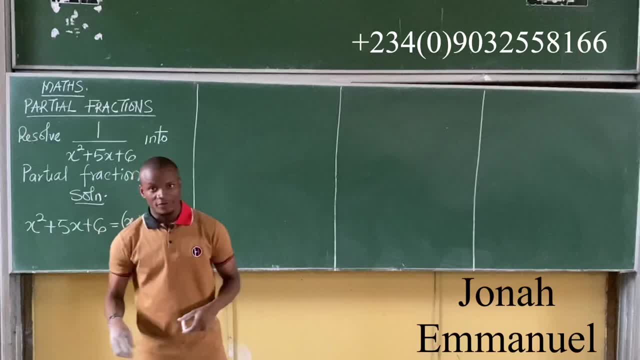 So this becomes the roots of this equation. X plus 2 and X plus 3. 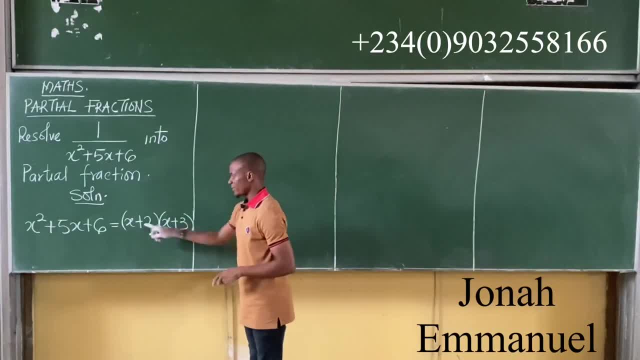 Now, observe that the roots are linear. Linear because the highest part, there is 1. The highest part of X is 1. So I have linear roots. 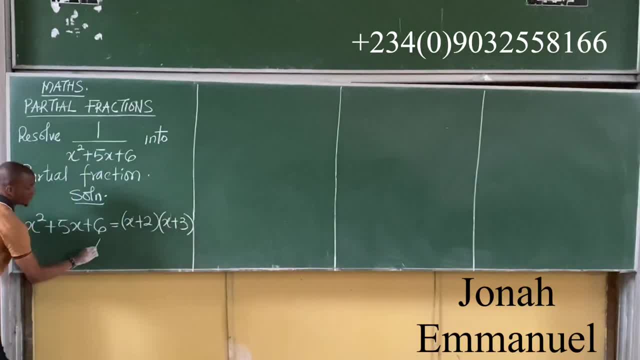 So we said for linear roots, a partial fraction of the form A all over AX plus B exists. So next up, after factorizing the denominator, your next task is to get the form of the partial fraction. 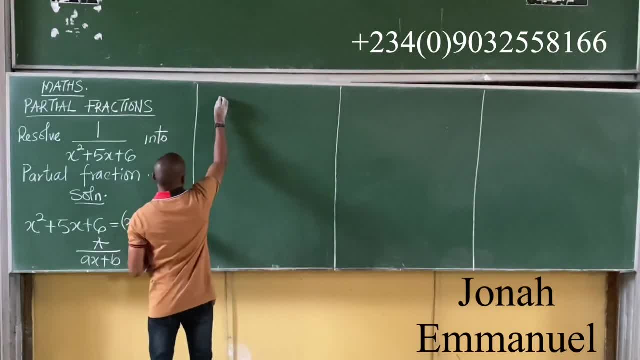 In this case, the form of this partial fraction would be 1 all over X squared plus 5X plus 6 would be equal to 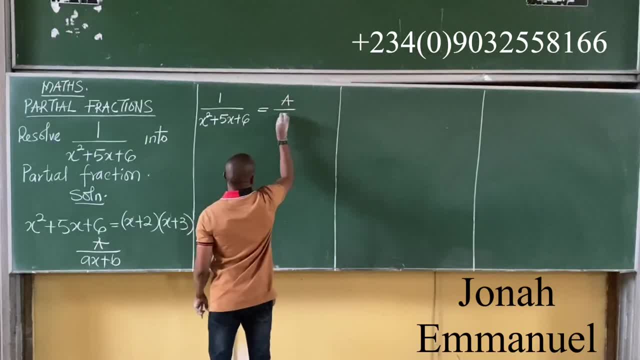 A over this first one there. That's A all over X plus 2. 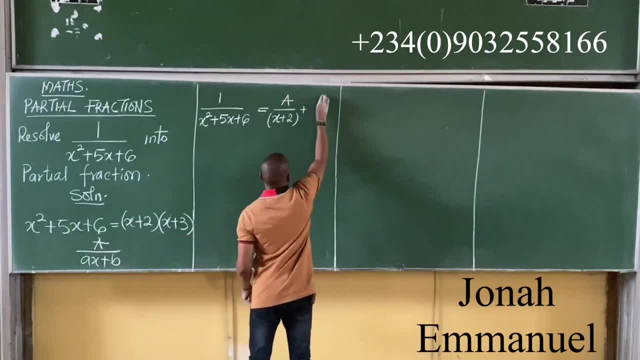 Next up, B to this. So plus B all over X plus 3. 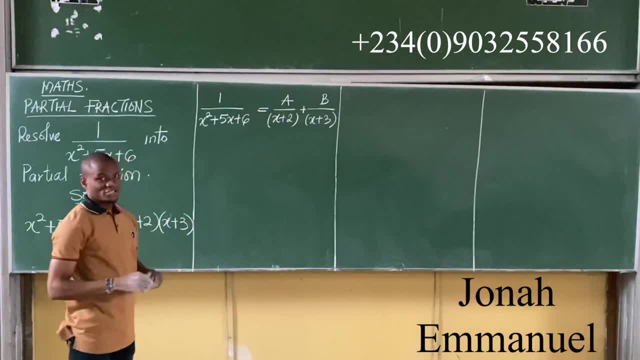 So this is now the form of this partial fraction. So after we get the form of the partial fraction, what next? 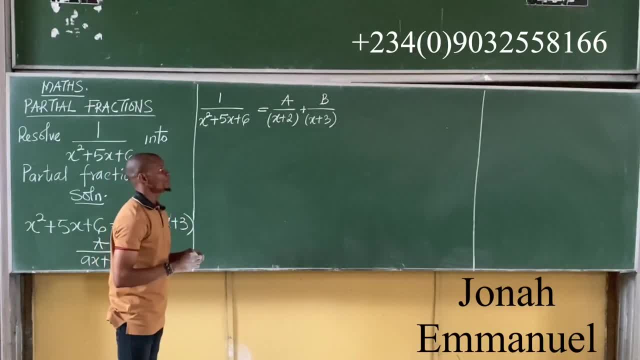 So after we get the form of that, my next task would be to take the LCM of these two. 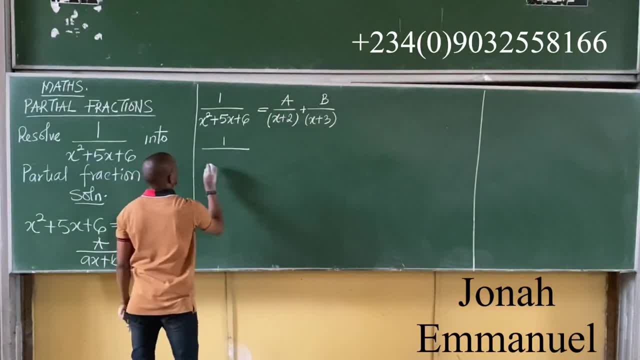 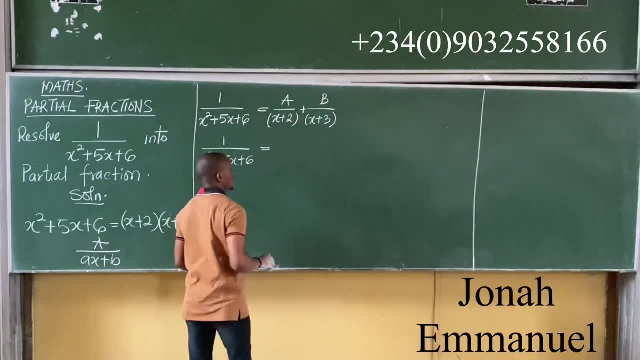 From here, I have 1 all over X squared plus 5X plus 6 is equal to Now, here's what I want to show you. Look at this. And here's what you should know. 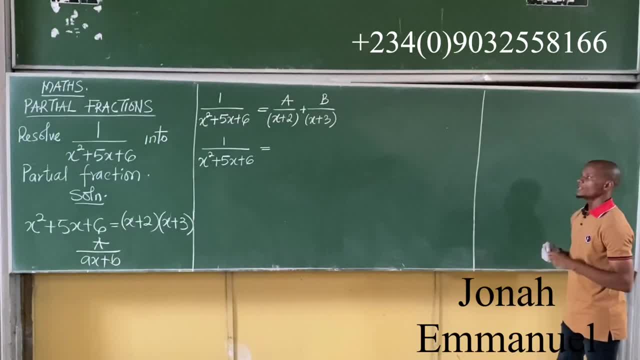 If I'm taking the LCM of, let's say, 2 on equal terms. Let's say 2 over 5 plus, let's say, 4 over 7 for instance. Of course, for this, my LCM is equal to 35. And of course, the surface becomes 35 divided by 5. It gives you 7. I'll use 7 to multiply this. 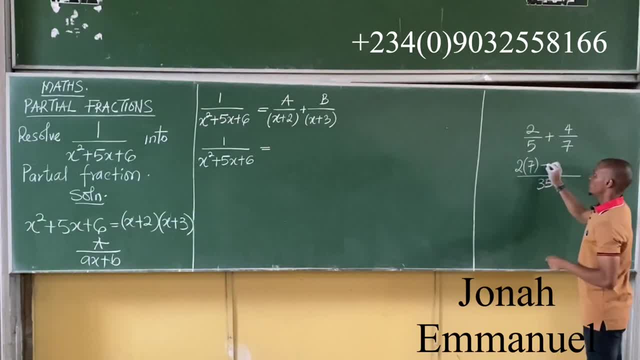 So it becomes 2 times 7 plus 35 divided by 7 gives you 5. 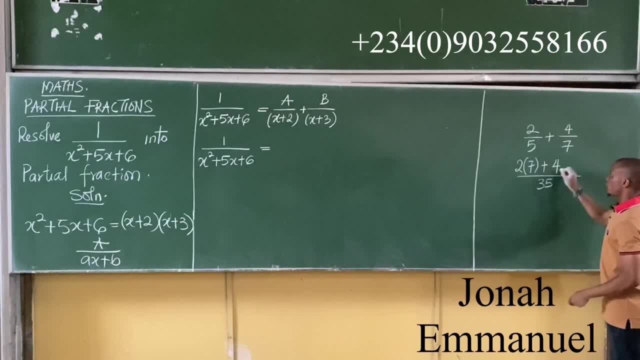 Use that 5 to multiply 4. It becomes 4 times 5. 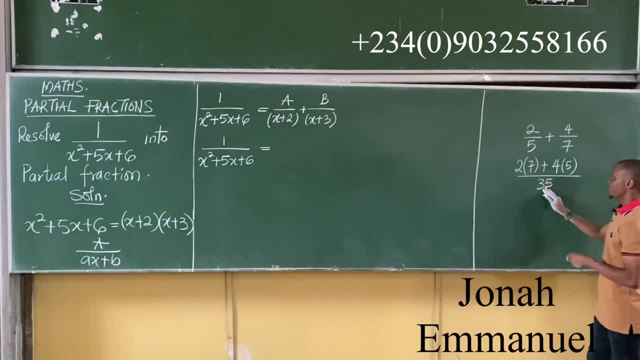 Now, here's what you should notice. 35 can still be expressed as 5 times 7. 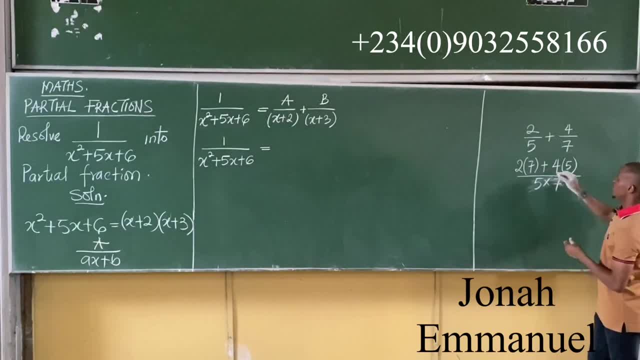 So the concept becomes this. If I'm having 2 uneven fractions added, we can say that the denominator is equal to the multiplication of these two denominators. So my total denominator here becomes to multiply these two. 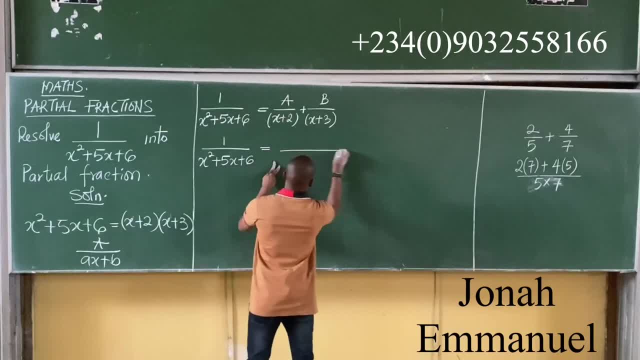 Use this concept here. It means that my denominator here would be to multiply these two. So it becomes x plus 2 into x plus 3. So we have this. Next up, also observe that this step here was what I had here, 2, multiplied by what I had here, 7. That's this times this. 2 times 7. The same idea will work here. 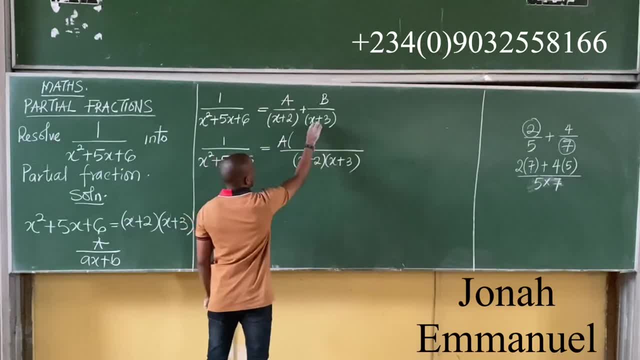 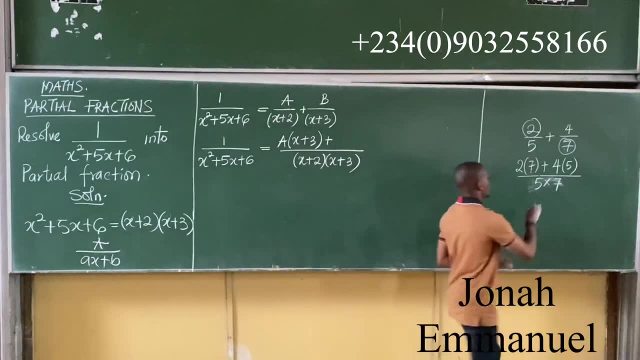 It becomes this one here, a, multiplied by what I had here, x plus 3. Next up, plus my next step here was what I had here, 4, multiplied by what I had here, 5, 4 times 5. So the same concept then becomes b, this, multiplied by what I had here, x plus 2. 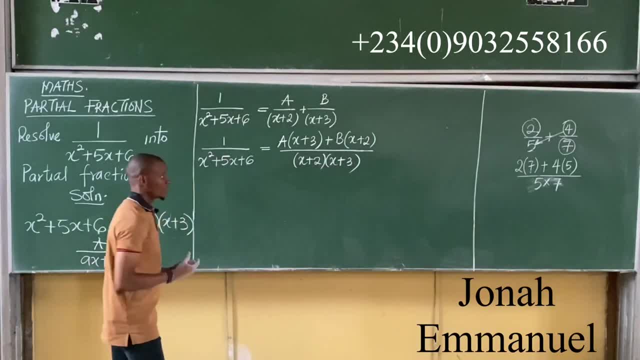 So I have these things. All right, so this is okay like this. This is how we solve. This is how we can easily work this out. All right, so what next here? At this point here, we can choose to equate numerators. At this point, we can equate. 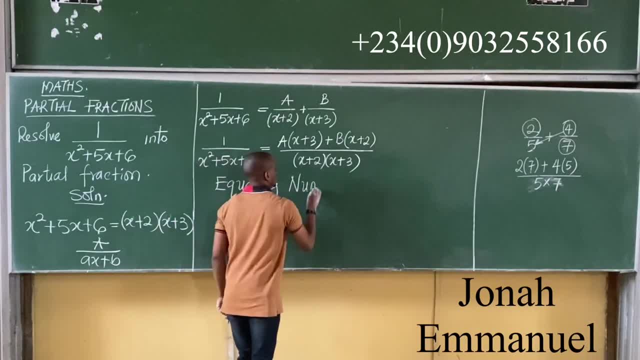 So equating numerators. Equating numerators. 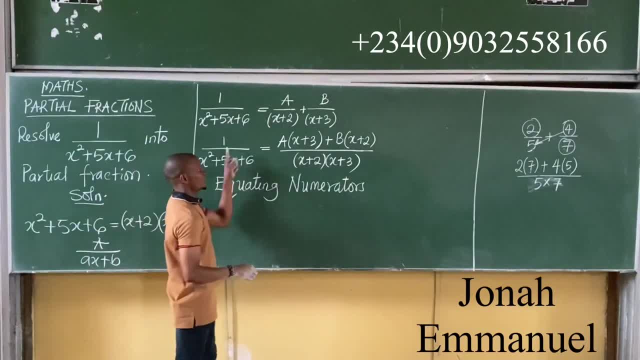 I have that over here. Now, we are equating numerators because the general numerators are the same. All right? If I expand this, I'll get this value. So since the numbers are the same, let's now equate numerators. 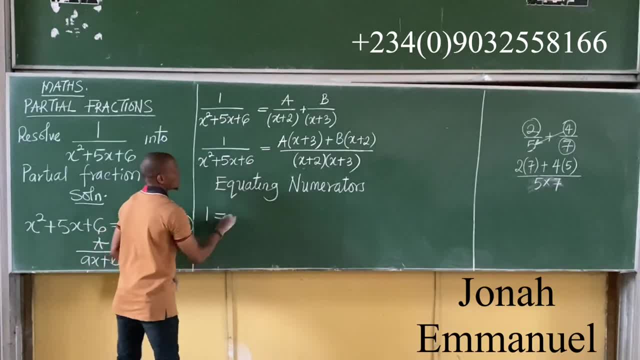 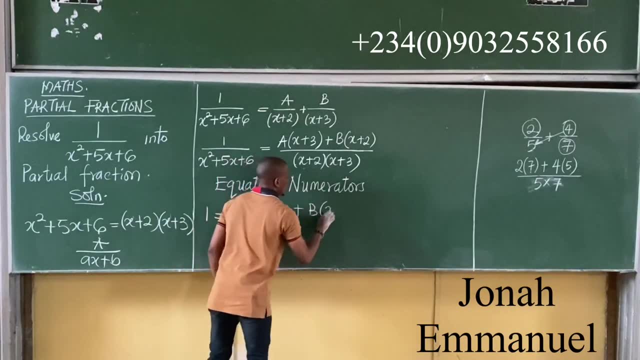 So it means that 1 is equal to, from here, I have a into x plus 3 plus b into x plus 2. 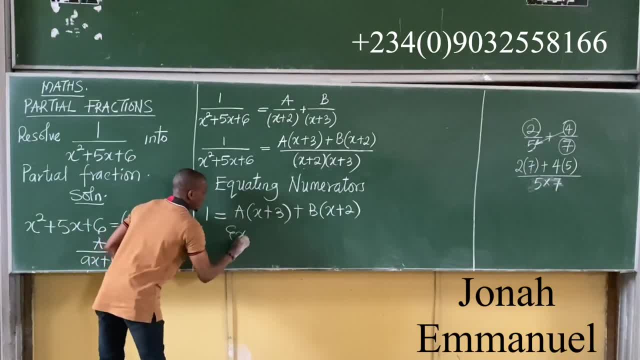 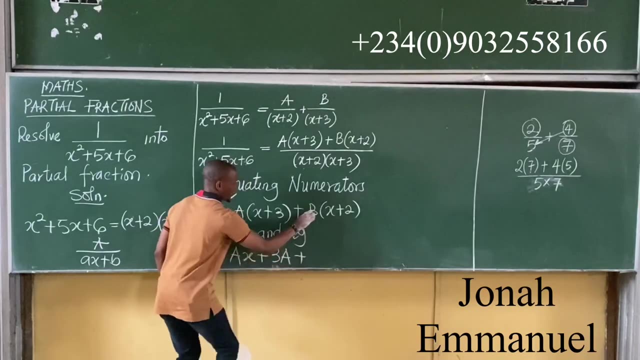 All right, from here now, I'll have to expand. So expanding, expanding, I have 1 is equal to a times x. It's a times plus a times 3. It's 3b plus b times x. It's bx plus b times 2. It's 2b. So I have this on expansion. 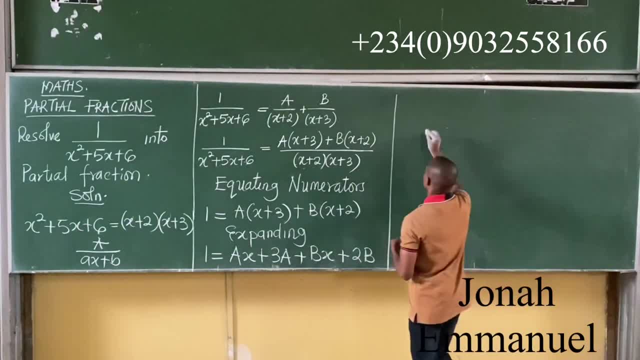 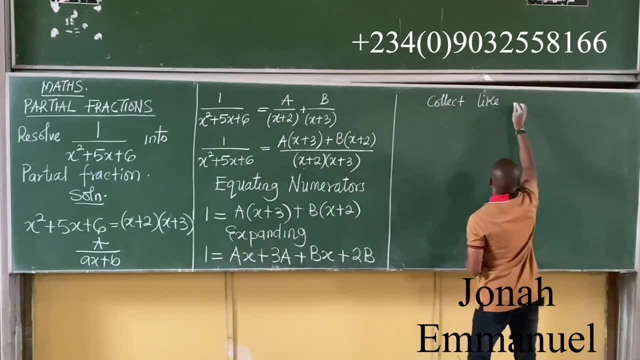 My next task here is to collect like curves. So I will collect like curves. 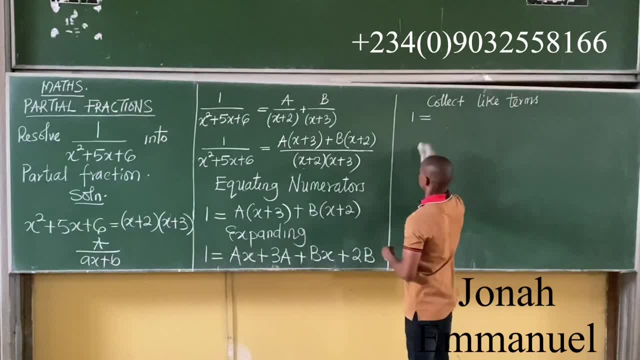 So 1 is equal to, for like terms, I will collect the terms having x. This one has x. This one has x. So ax plus bx. I'm having ax plus bx. I'm done picking the terms that have x. 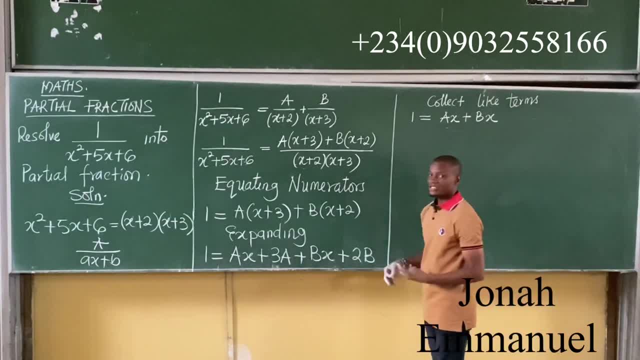 Next up, take the constant terms. Constant terms are simply terms that do not have x. That becomes 3a plus 2b. 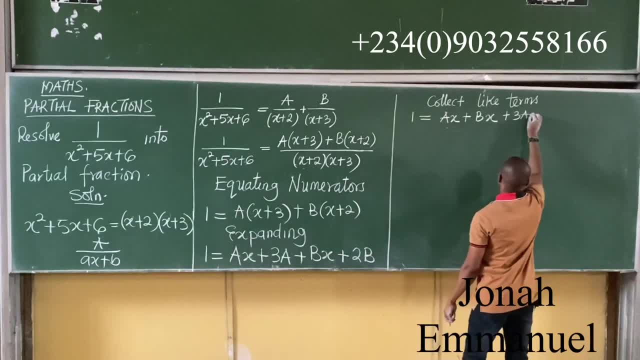 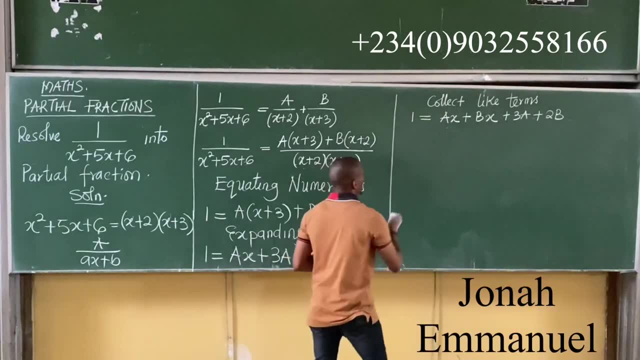 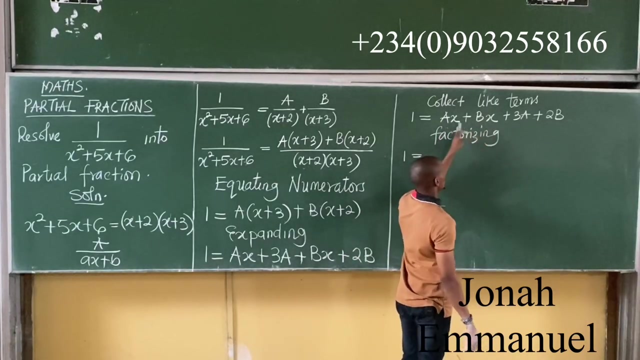 So I have plus 3a. Next up, plus 2b. After collecting like terms, what next? I'll have to factorize, factorizing. If I factorize this, I have 1 is equal to, these two terms contain x. So factorize the x out. If I take out x here, I'm left with just a. Take out x here, I'm left with just b. So it becomes a plus b. 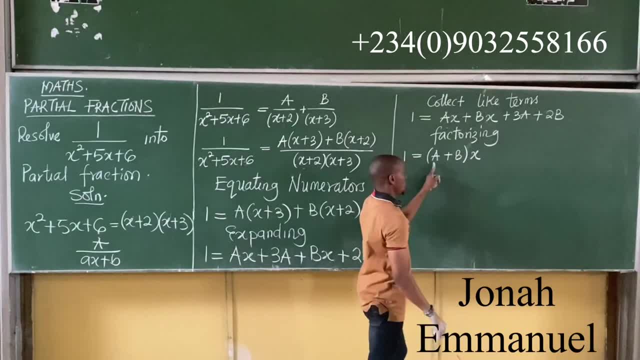 This all equal x. So a times x gives you ax. b times x gives you bx. Next up, take out the constants. 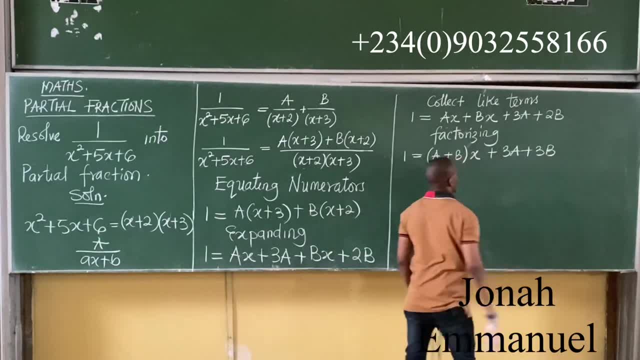 3a plus 3b. I have this. Alright. 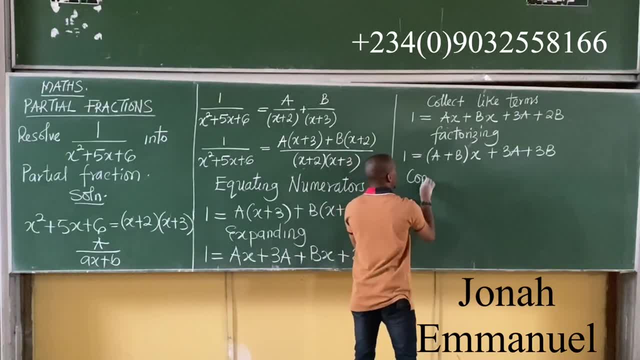 After factorizing, next up, I'll have to compare. Or you can say, comparing. 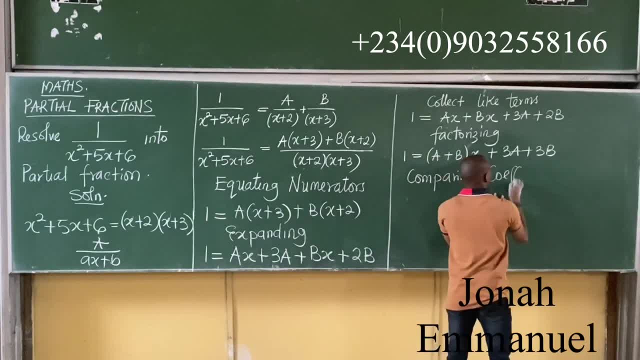 Comparing coefficients. Coefficient. 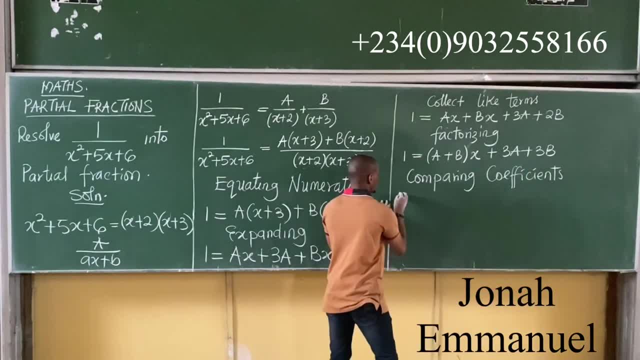 Comparing coefficients, I have this. First of all, the highest power of x here is 1. So I have of x. If I look at the left-hand side, from here, there is no x here. That means the coefficient of x here is 0. So I have 0 is equal to. From my right-hand side, the coefficient of x becomes this one there. That becomes a plus b. Call this your first equation. 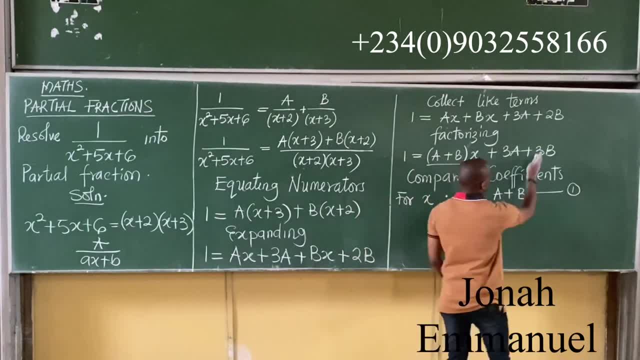 Having a plus b. This was 2b. Okay? So plus 2b, please. That was 2b. Alright. Next up. After x, I have this one as constant. 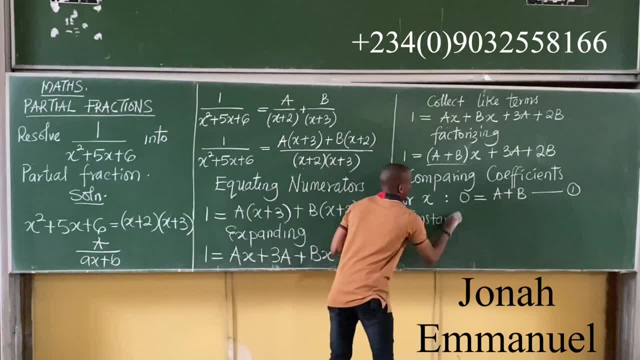 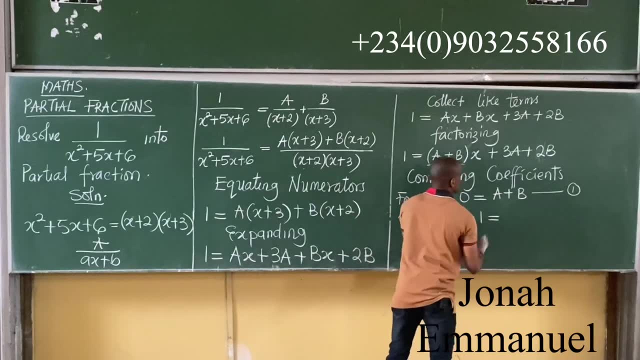 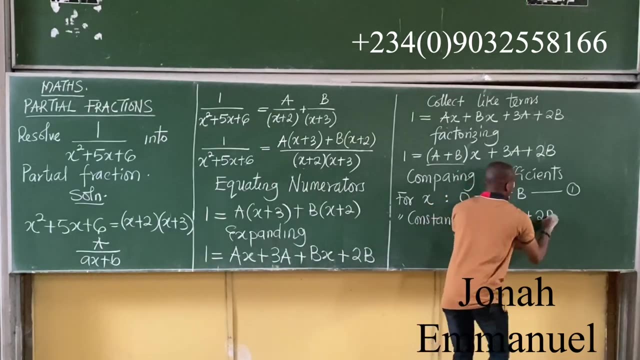 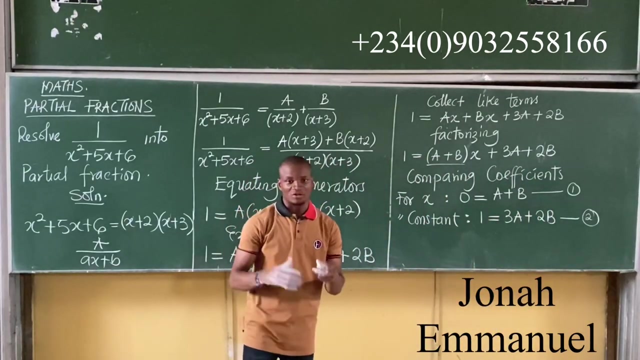 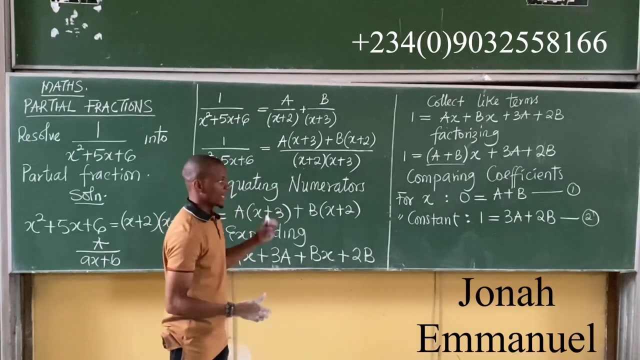 2 of 4. For the constant, what do I have? On my left-hand side, my constant is 1. So I have 1 equal to. For right-hand side, my constant is 3b plus 2b. Call this equation 2. And I have two equations. Equation 1 and equation 2. I'll have to solve equation 1 and 2 simultaneously to get the value of a and b. Alright. 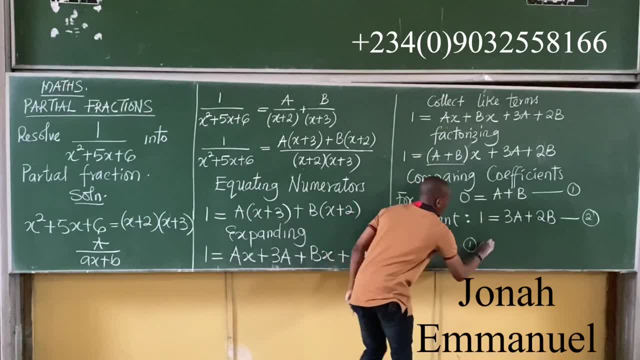 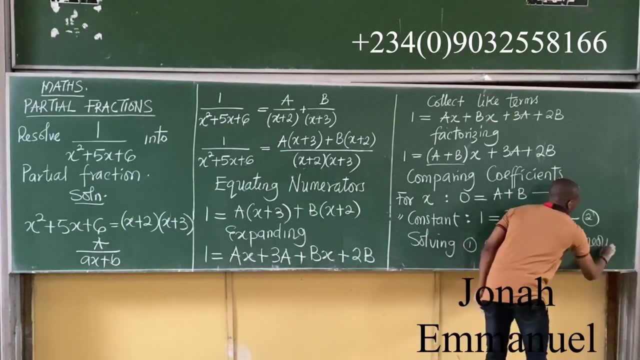 So solving equation 1. And 2. Simultaneously. What do we get? Alright. 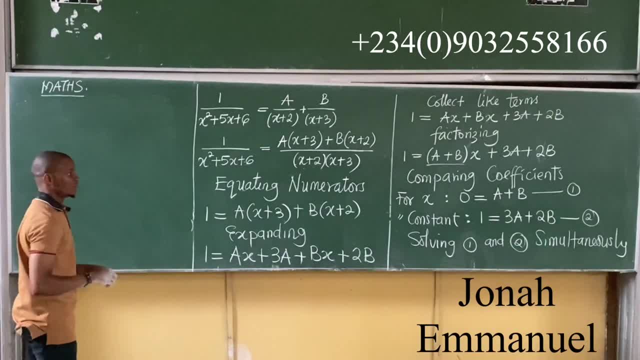 So I've solved it using the ideal substitution method. From substitution method. From 1. 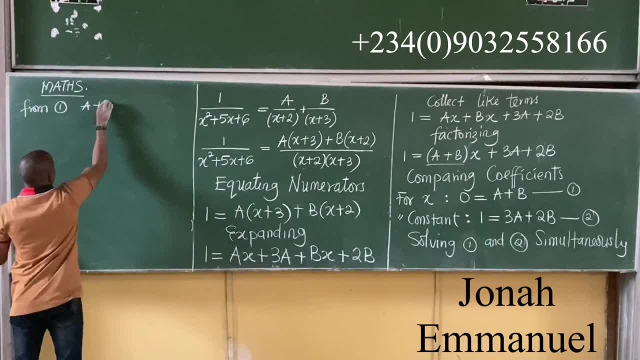 From equation 1. We said a plus b is equal to 0. 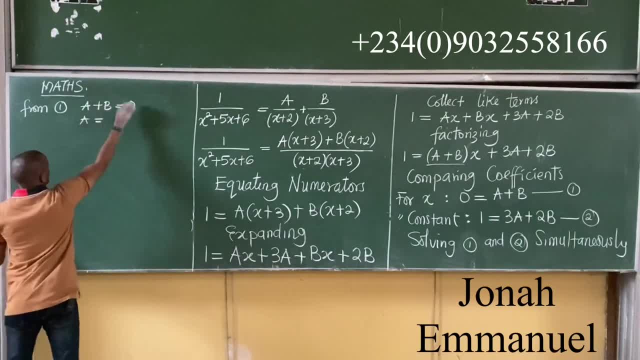 Move the over here. So a is equal to. 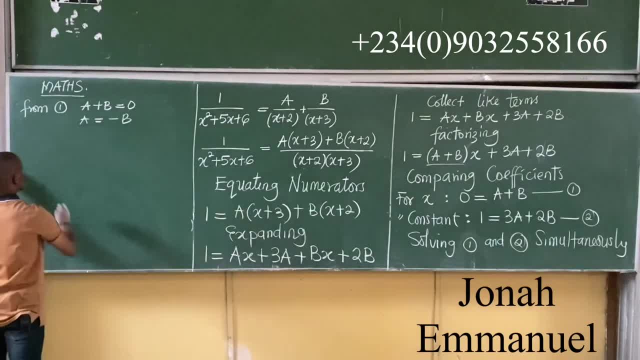 Now the answer becomes negative b. I'll put a as equal to minus b into the other equation. That's equation 2. Into equation 2. And that gives 1 is equal to 3a plus 2b. 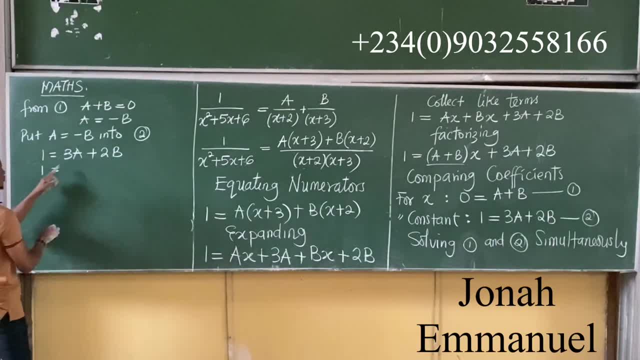 Fix a here. I have 1 is equal to 3 into a. a is minus b. Then plus 2b. From here, it means that 1 is equal to. 3 times minus b is minus 3b plus 2b. From here, 1 is equal to minus 3b plus 2b is minus b. To get b, divide here by minus 1. Divide here by minus 1. This cancels this. 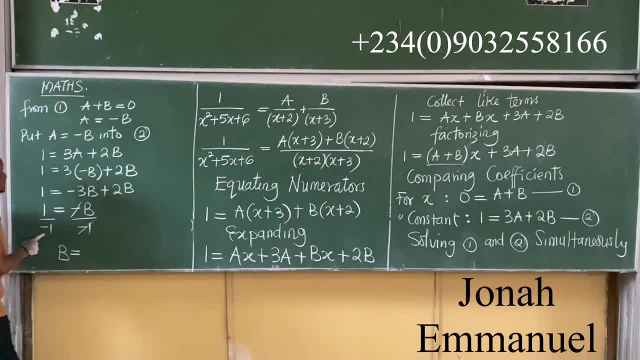 So it means that b is equal to 1 divided by minus 1. Gives minus 1. Subtract the value of b as minus 1. Let's get the value of a. From here. From this equation here. We said that. We said that a is equal to minus b. 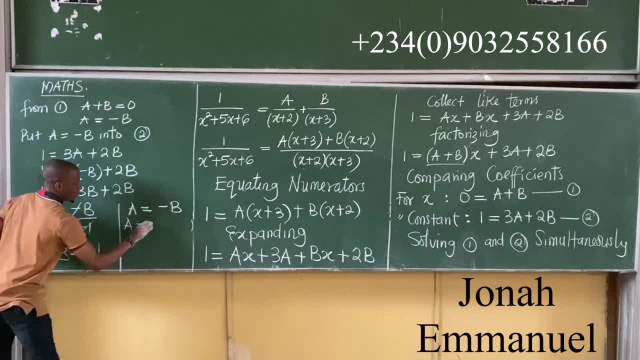 That means a will now be equal to minus b is minus 1. Because minus minus 1. That means a is equal to minus minus 1 is plus 1. So a is 1. Why b is minus 1. So I have a as 1. And b is as minus 1. Alright. So if you got the value of a as 1. 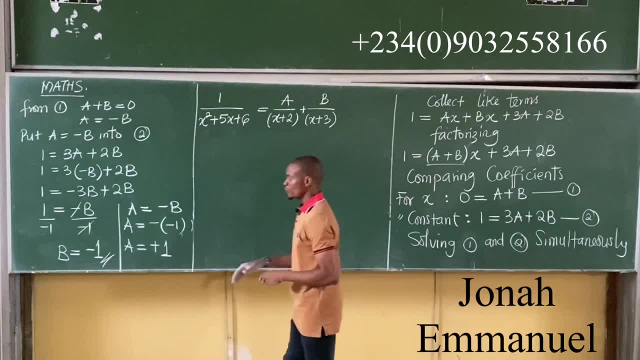 And b as minus 1. And that allows me to put the value of a and b back into a general form. 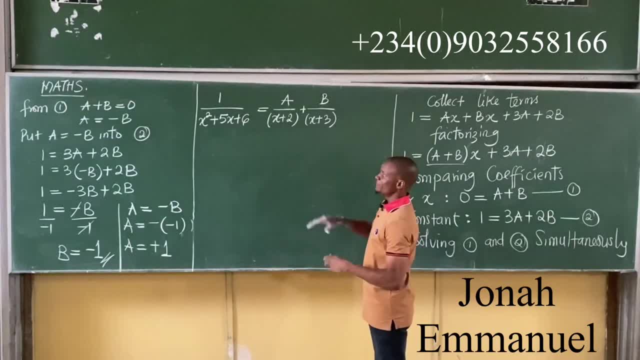 Now recall that this was a general form of the partial fraction expression. So therefore, put the value of a and b here. 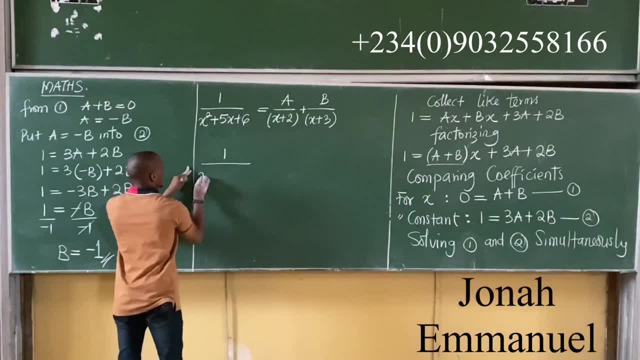 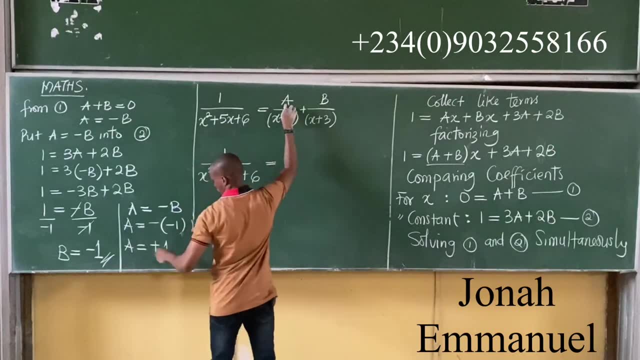 This now is 1 all over x squared plus 5x plus 6 is equal to a. a we said is plus 1. That becomes 1 all over x plus 2 plus b. So this is minus 1. That becomes minus 1. 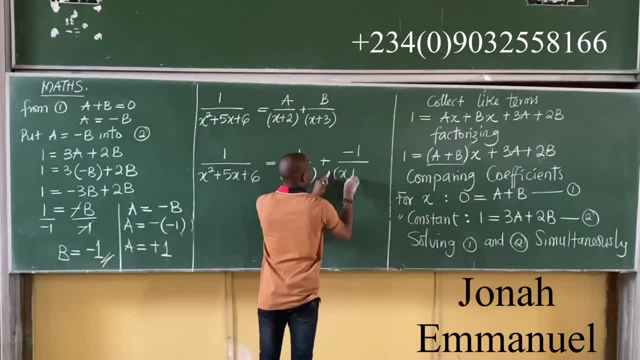 That becomes minus 1 all over x plus 3. So we have this answer. 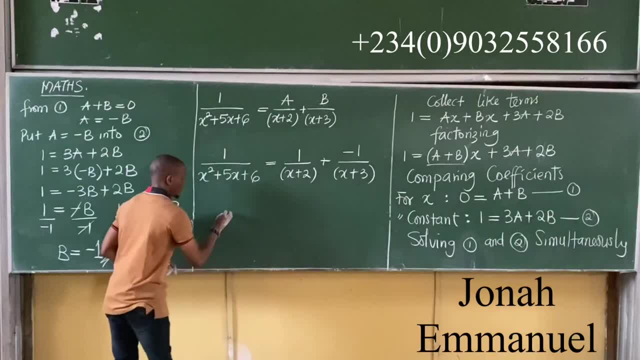 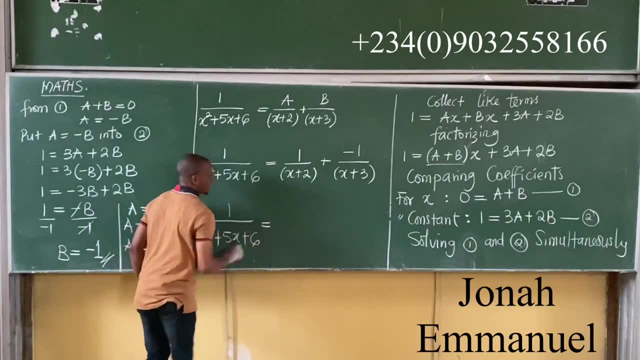 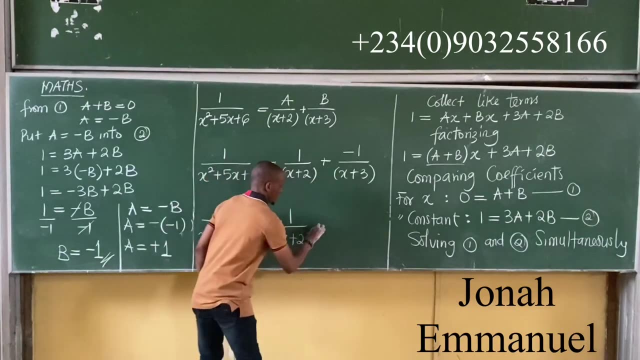 Next what we have is to define this. So that means we have that 1 all over x squared plus 5x plus 6 is equal to 1 all over x plus 2. Plus minus is minus 1 all over. So this now becomes my final answer after solving. 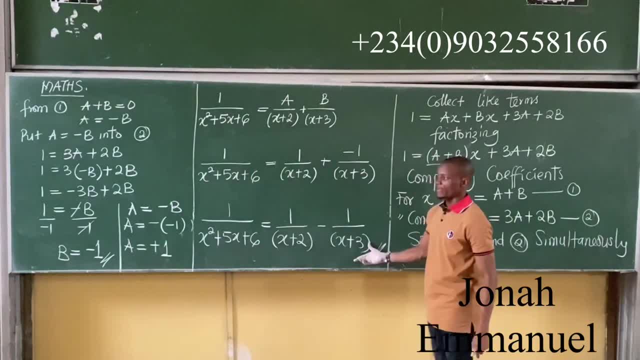 So this is how you resolve this into partial fraction using reward. So this is the answer. Alright. 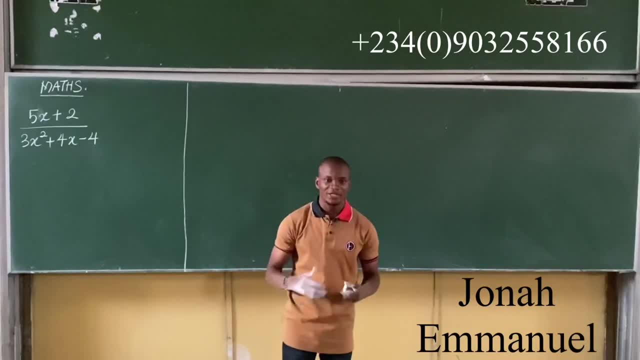 So let's solve a second example on partial fraction. 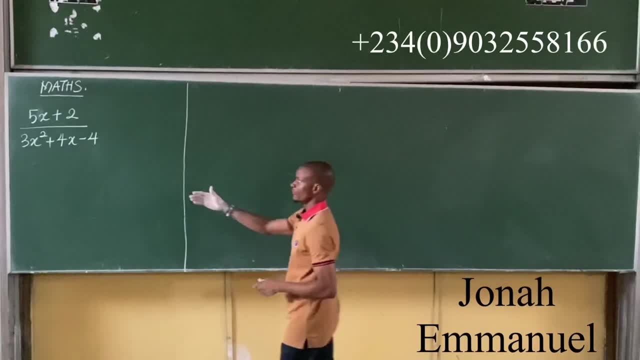 So let's say that we are given to resolve this into partial fraction. So as I said. 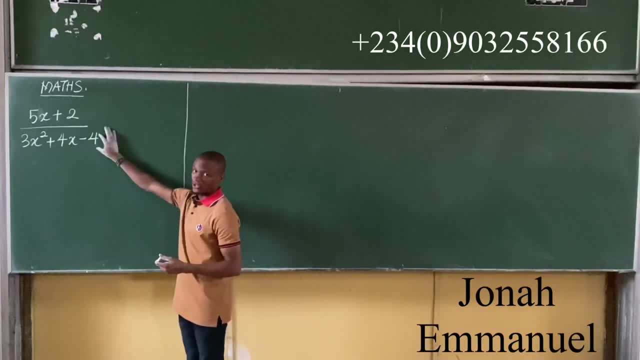 Your first task is to always consider your denominator. In this case, the denominator here is 3x squared plus 4x minus 4. This is a quadratic equation. And if I resolve this one here or if I factorize this using the ideal quadratic equation. This will give 3x minus 2 into 2x plus 2. In our previous classes we looked at how to evaluate quadratic equation by factorization method. Alright. If you have not checked it out. 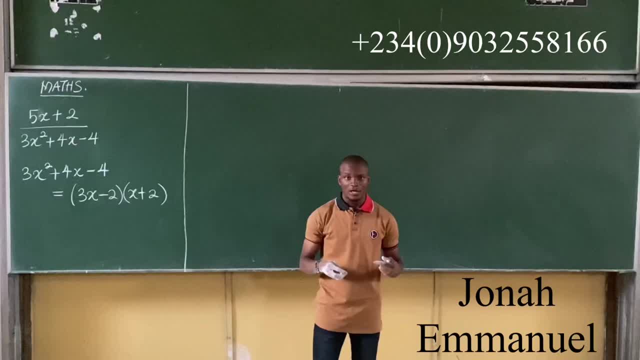 Just check out the video in the link that we provided in the description of this video. Just go to the description of this video. You will see a link provided on how to solve things like this with factorization method. Alright. 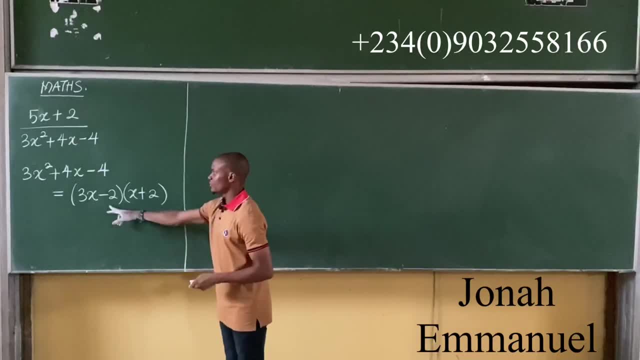 So let's proceed with this now. So if I look at this. I now have the two rules of this equation. 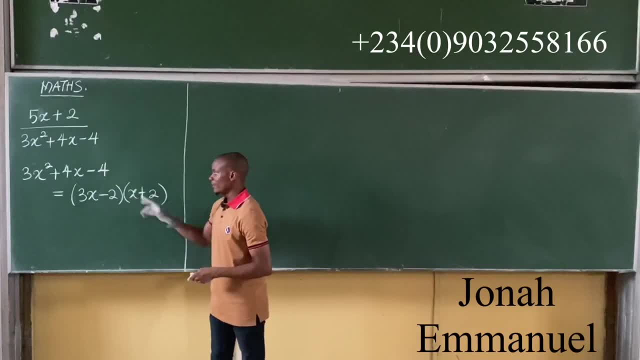 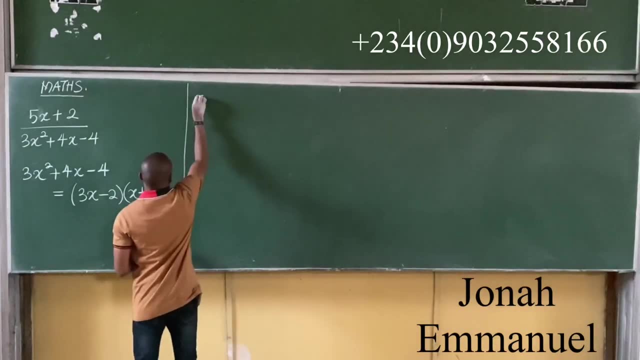 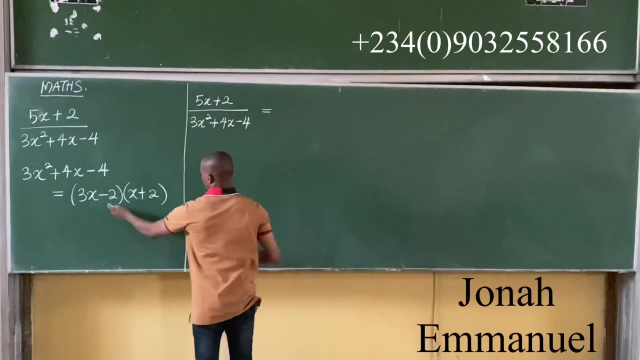 And of course these are in linear form. So of course let's now get the form of this partial fraction. So this will now be 5x plus 2 all over. This is 3x squared plus 4x minus 4. This will be equal to. a all over this. That's a all over what I have here. This is 3x minus 2. Plus b all over this one here. 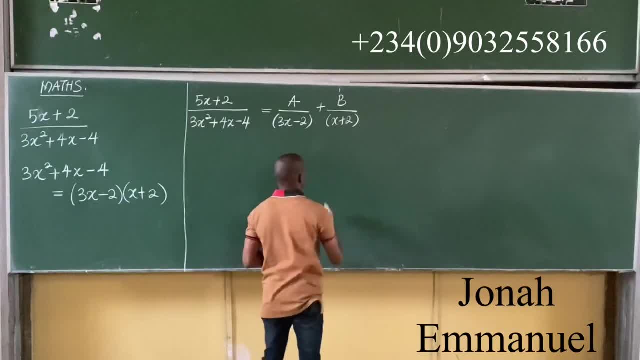 This is x plus 2. So this now becomes the form of quadratic equation. 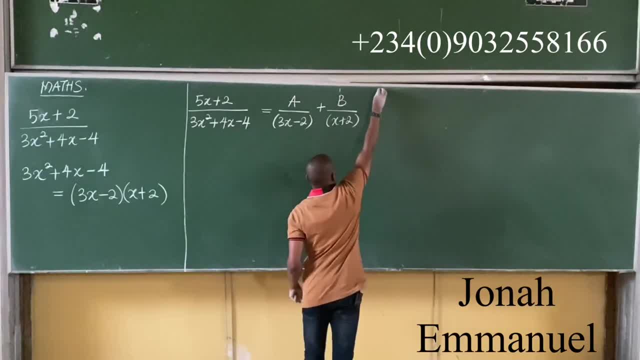 My next task here is to get the else here. So from here. 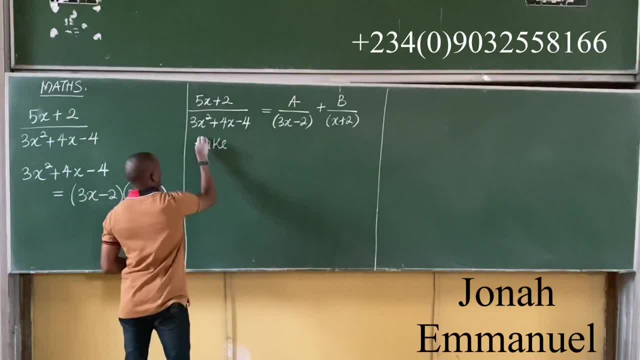 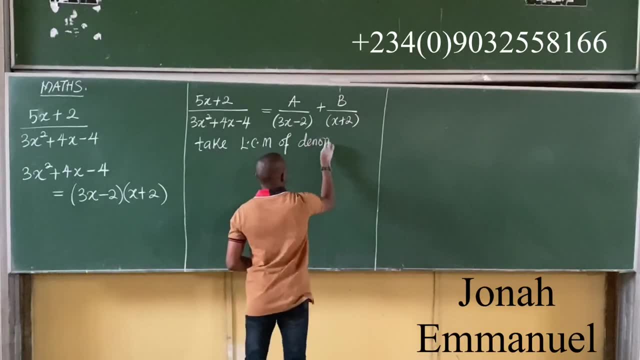 I will take the else here. Of denominator. If I take else here. 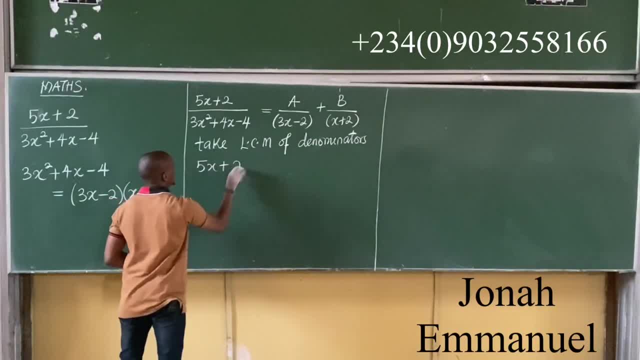 This gives you 5x plus 2 all over 3x squared plus 4x minus 4. Equals. So we said from our first example. We said. 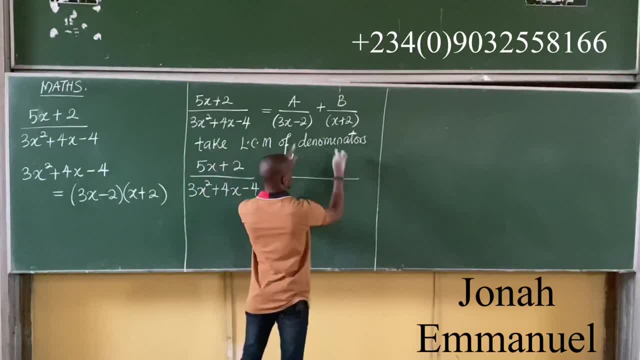 Your denominator is usually. This 2 being multiplied. That will be. 3x minus 2. 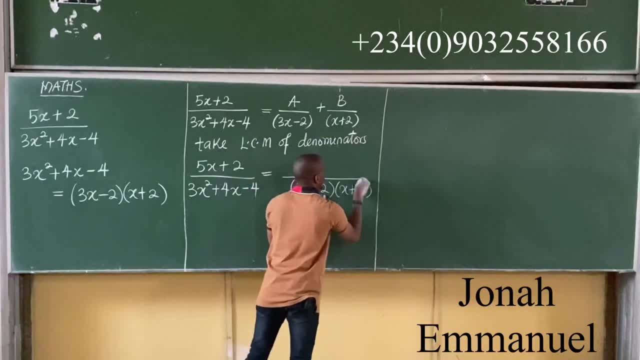 Multiplying. x plus 2. So the next task. 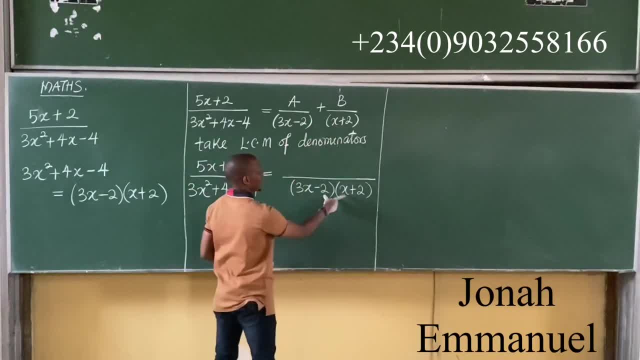 This will now multiply this. Because divide this. Divide this one here. With 3x minus 2. 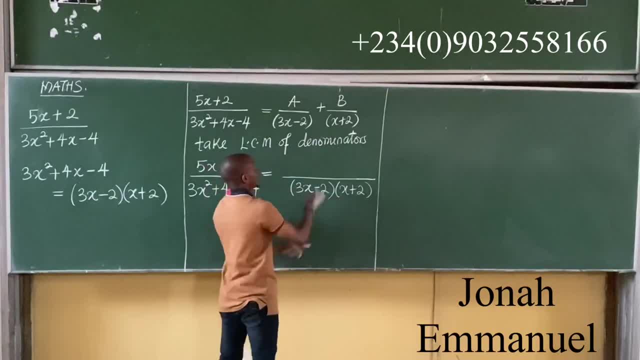 This will count to this. 11x plus 2. Then x plus 2. That number comes in. Into. x plus 2. Next up. Plus b. So I'm having. Plus b. Into. 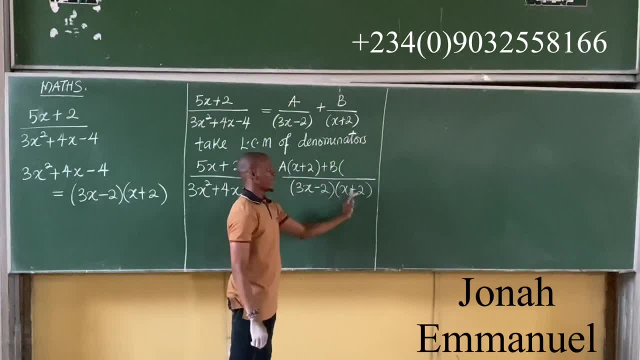 Divide this with this. So x plus 2. Counts to x plus 2. 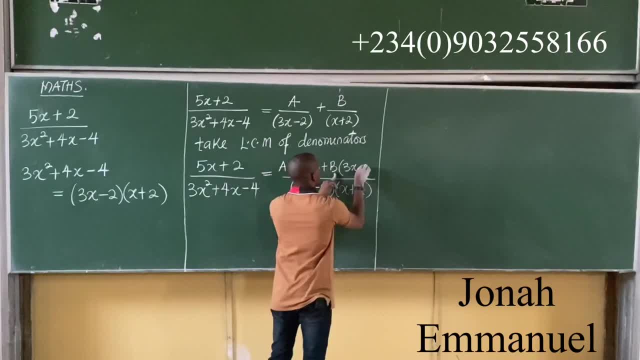 And that is 3x minus 2. So 3x minus 2.